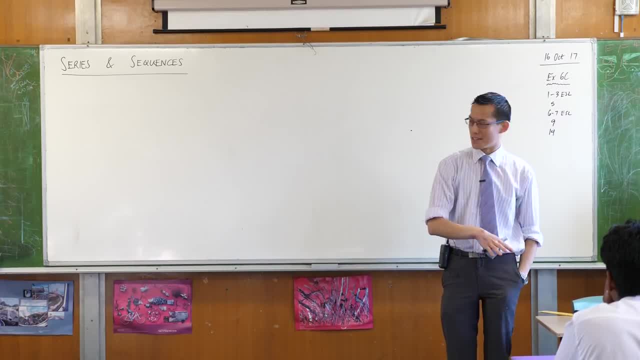 However, it goes some really, really important places. So it's not as though things are getting easier. It's just a temporary break for your brain while we get you going for the next thing. So this is the heading. There's the date. Got this down already because I was a bit more organized today. 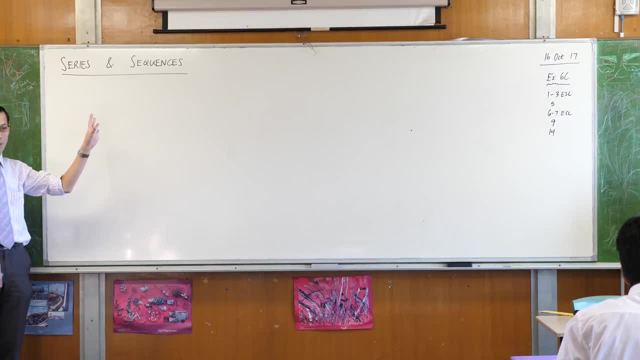 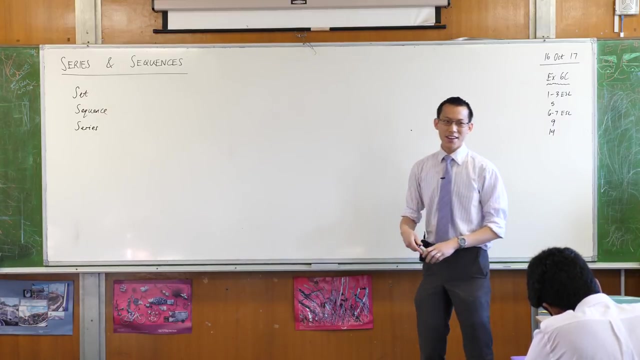 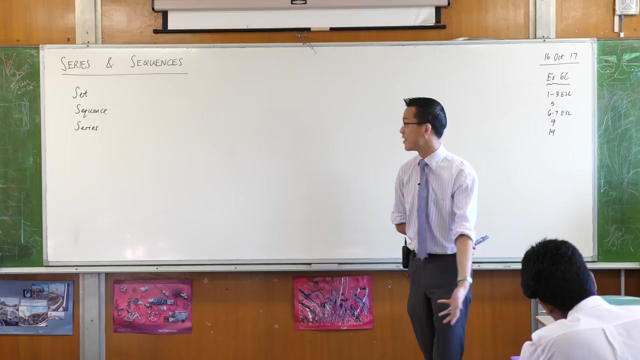 We are interested in a particular kind of new object, Actually a whole bunch of them, that are related together. There are three, and I'm going to explain them in order, which, as you'll see, in a second. In a second is quite ironic. So, even though it's not in the title here, the best place to start in this topic is with an object, a mathematical object, called a set. 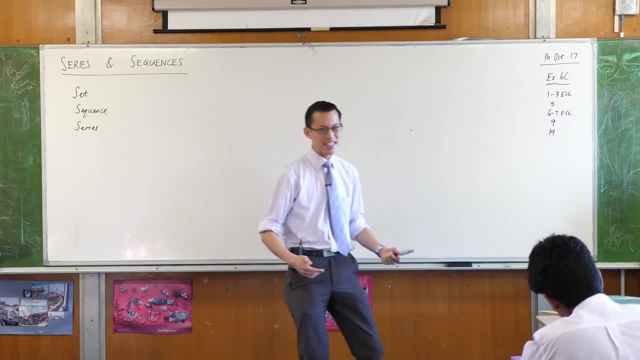 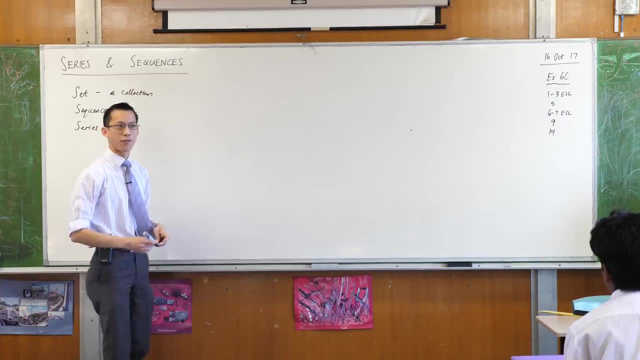 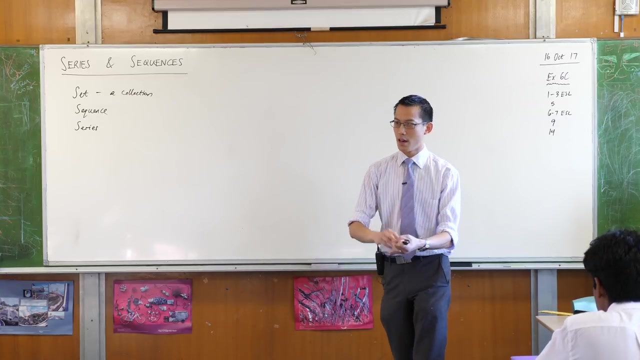 It's a really, really simple kind of object. All it means is you collect a bunch of things. In fact, a collection is a good way to define or a good synonym for a set. You've got a bunch of items. They could literally be anything. They could be a bunch of numbers, a bunch of functions. 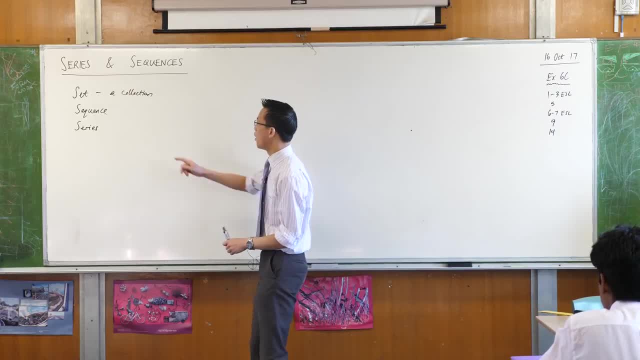 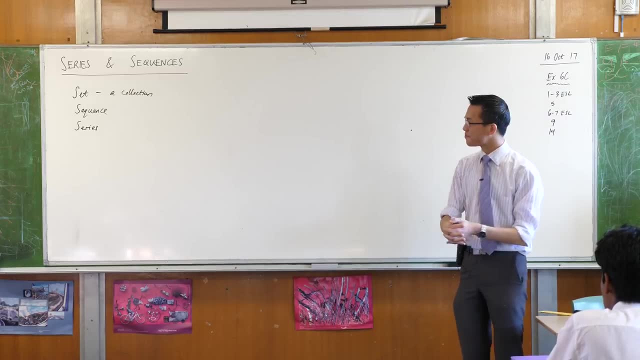 A bunch of shapes, Anything you want. All that matters is that you've got a bunch of them and you put them in a big pile. That's what a set is. Now where it starts to hit. the rubber hits the road for this topic is when you say: 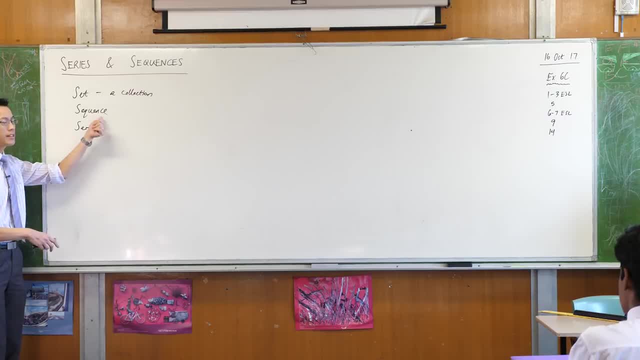 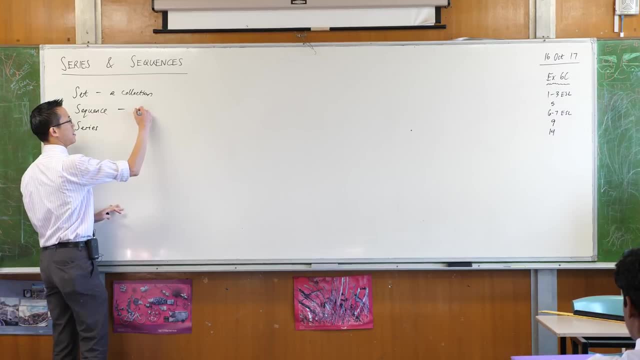 well, let's take that collection of things and let's put them in some kind of order. So a sequence is a set that has an order to it, A set with order. So, for instance, here's a set. It's a black marker and a red marker and a blue marker. 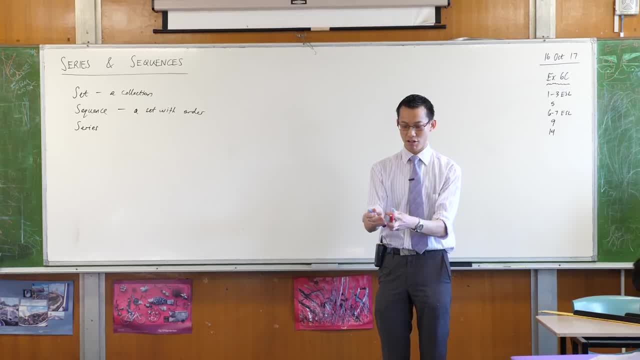 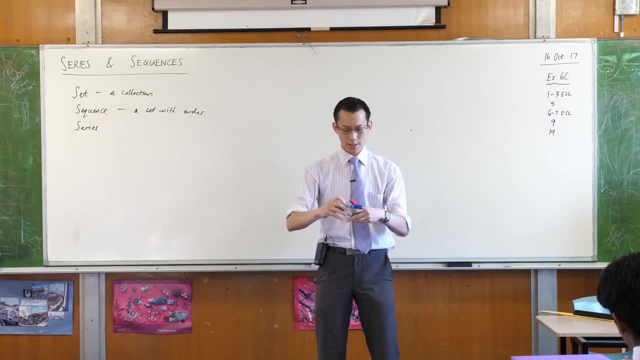 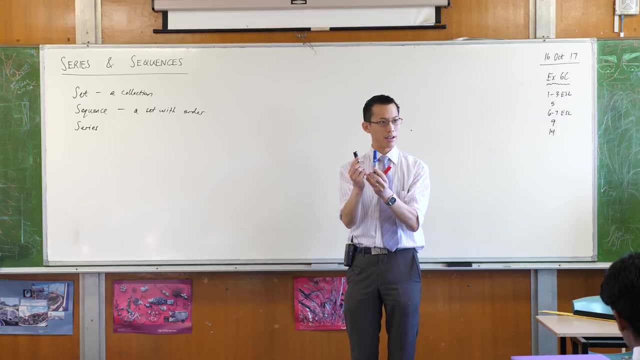 Here's a set. No matter which way you look at it, it's still the same set. Nothing's changed. But for me to say: okay, let's make a sequence of markers. This sequence here- blue, black and red- is different from this sequence here: black, blue and red. 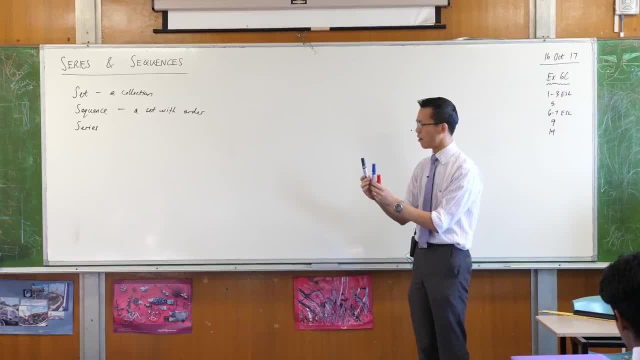 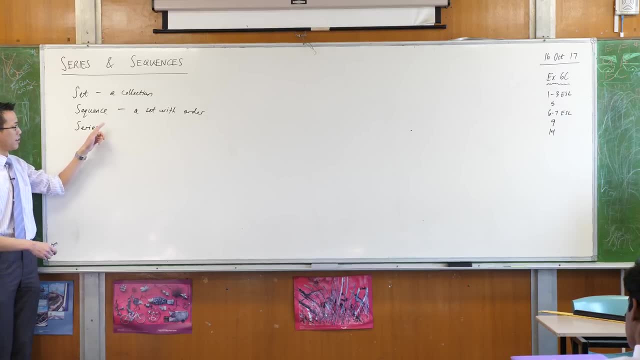 Right. So all that matters here when we talk about sequences, is all right. now it matters which order I place these in, And that's what makes this a sequence. We're not going to get into a series until a little bit later in this topic.